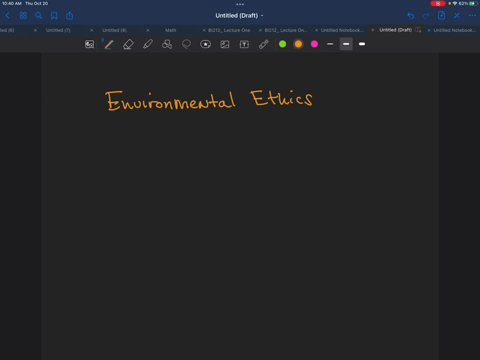 It's a form of philosophy. It's an idea of how we view the world and what we see as being right or wrong, or good or bad. When we talk about environmental ethics, it has to do with how humans view good and bad, as it is related to their relationship with the environment. 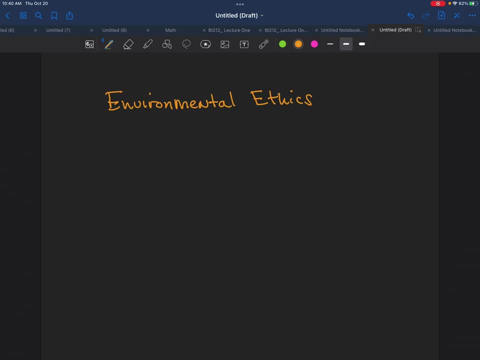 So this has a lot to do with your biases and your worldview. So, for example, if you are from a very rural area and you are from a place that animals are used to as a form of say, for example, business transactions, then you probably see the world a lot differently than if 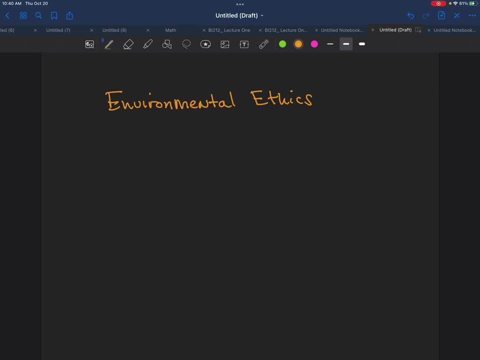 you live in the city, where you are removed from the land and removed from the business of producing animals, say, for example, with for human consumption. And that is not necessarily right or wrong. It just is that we all have different worldviews and we all have different values, and just acknowledging those differences 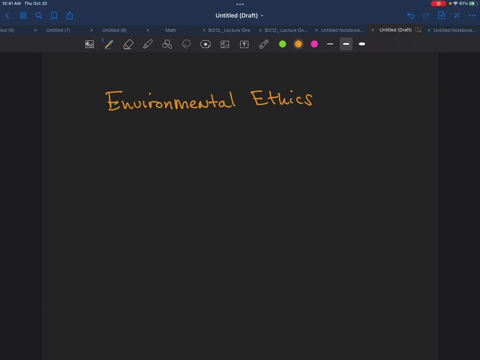 is important. When we talk about the value of nature and the natural world, there's two different ways that we can value it. One is what is referred to as its instrumental value. So this would be how it is useful to us. So this is this idea of utility, So this is a utilitarian. 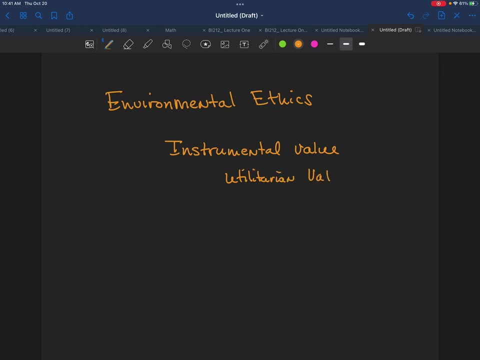 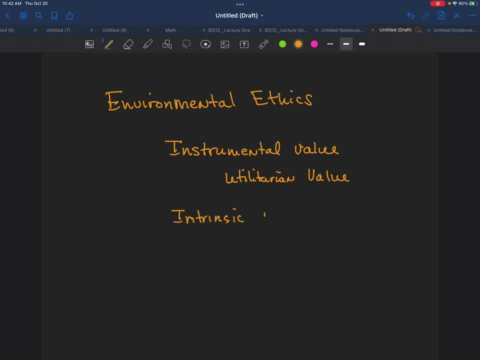 value. So this is a utilitarian value And this means that we could have an inheritance value for that land. But thesten of you can probably not define this. is intrinsic value, just the proprio unused value or its inherent value. So you might also believe- and it can not just necessarily. 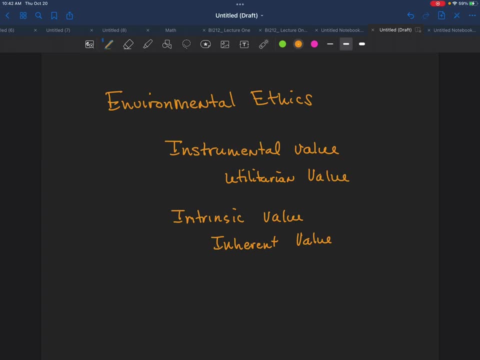 be one or the other. but you could also believe that forests have a value outside of what humans can do with those forests, of what humans can do with those forest. so there's a value that could be applied, that's an inherent value That gives. yeah, I guess. 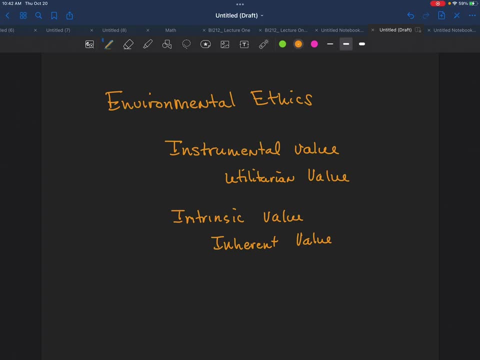 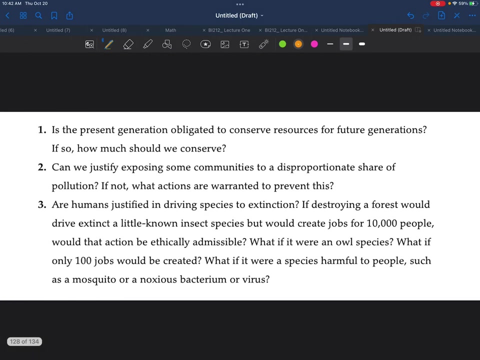 the idea that it might be wrong to to clear-cut all forests and all old growth simply because there is an inherent value to it that is outside of what you can extract from it. So these are two different ways that we might value the natural world. This gives us different world views, So we can talk about ethics. 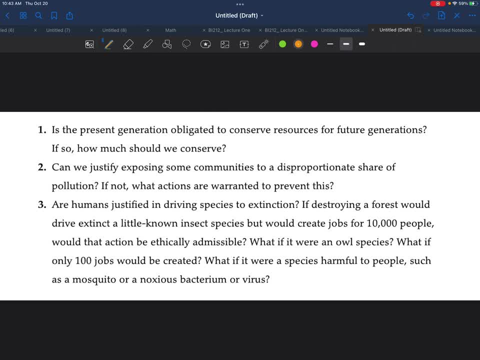 and also what is good or wrong. So we might also think about how our present generation is using resources and if it is bad that future generations are not going to be able to have the same bounty that we have currently. We might also talk about whether it is good or bad to have certain populations certain 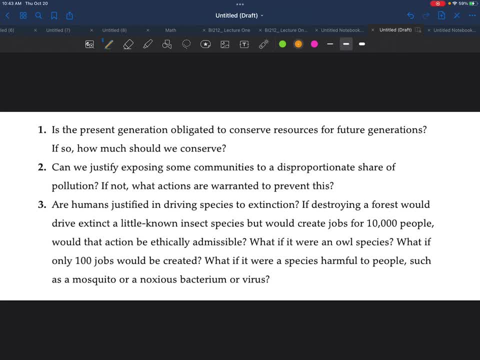 communities that are disproportionately unpopular, So, for example, people that work in agricultural fields and are more subjected to the insecticides and the herbicides and how that might influence their health, And so that's also part of what we call environmental justice. Is it okay for us to drive species to extinction? So if there's just like this, 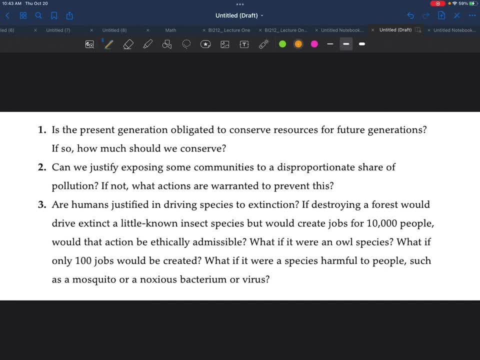 one species that is in the way of using a forest for logging. is it important that we conserve that one species rather than log the forests? And how many species are important? Is it more important to value vertebrates, say, for example, over invertebrates, so like owls versus slugs? 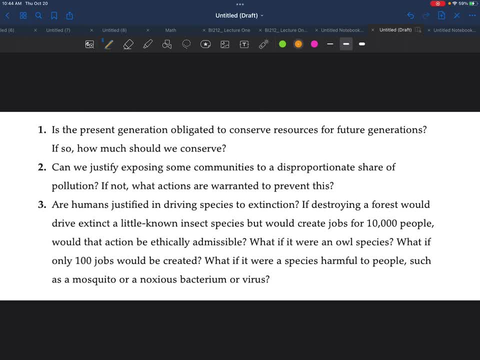 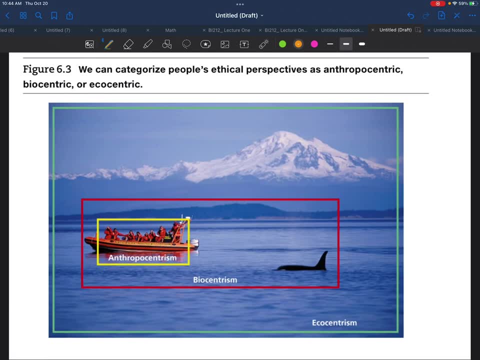 when we look at that, And so these are all part of this, what is referred to as environmental justice, environmental ethics. One way that we can also look at our worldview and our point of view is through these different lenses. This first one is called anthropocentrism, and this is the idea. 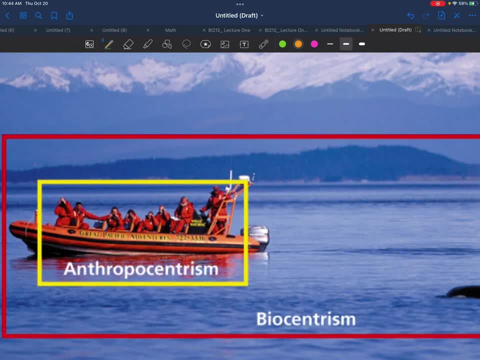 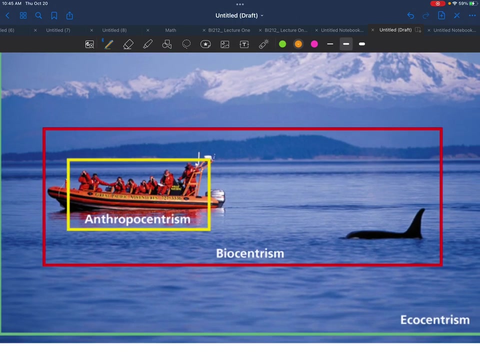 that nature. we are outside of nature, and nature is something that is useful to us, but we are not necessarily a part of nature, And so valuing things because they can provide humans something would be one way of viewing the world. The other way would be taking into consideration other 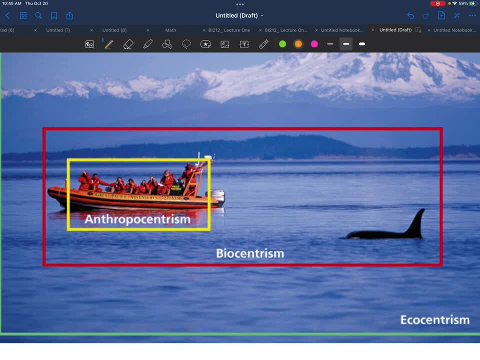 species. So maybe you have a biocentric viewpoint and it's important to realize that oftentimes we are more attracted to the high profile organisms like killer whales and whales and, you know, maybe even the furry animals, say, for example: 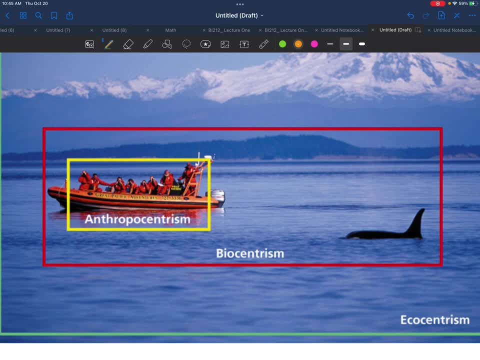 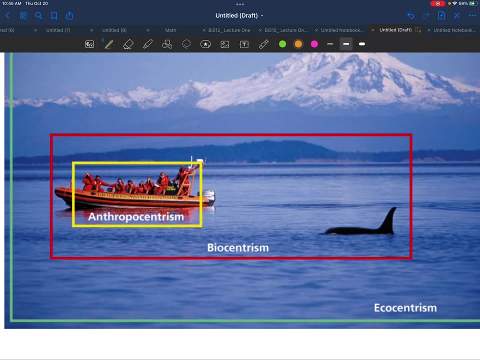 lions and bears and stuff like that in terms of conservation, And so we might have a limited view of this in terms of just looking at species conservation. And then there are people that are more ecocentrism, which means that we should be focusing on the preservation of entire ecosystems, So not. 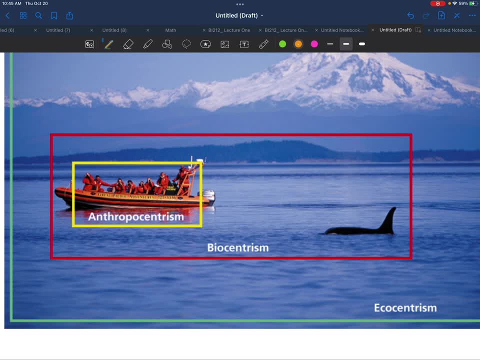 just the without the rhizomes. So what I'm trying to get at is: why are we able to have a climate? the living parts, but also the non-living parts. So the entire Puget Sound, for example, is important to conserve parts of that, to have parts of that being conserved, just because of the intrinsic 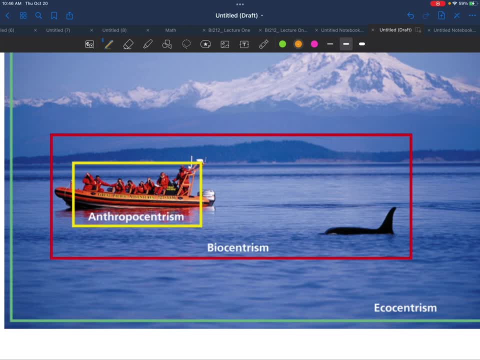 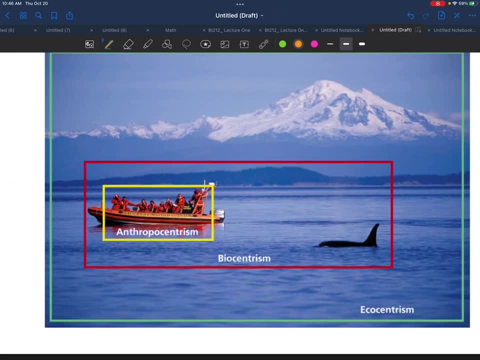 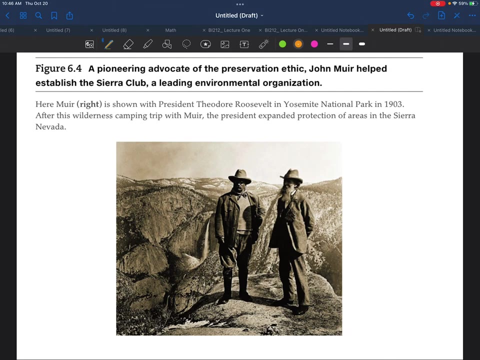 value of it, as well as the economic value that it might provide in terms of ecosystem services. Now, there are two famous people that have kind of different histories. One of them is John Muir, who was around at the same time as Teddy Roosevelt, our president, who created a lot of 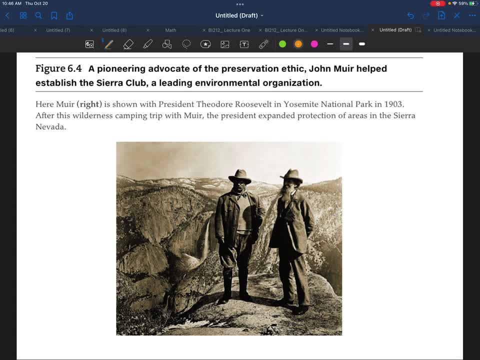 national parks And his idea was to set aside land and preserve it. So he had what is referred to as the preservation ethic. So this is a preservation ethic- Preservation, So this has to do with wilderness. Are there places where we should not have motorized vehicles? 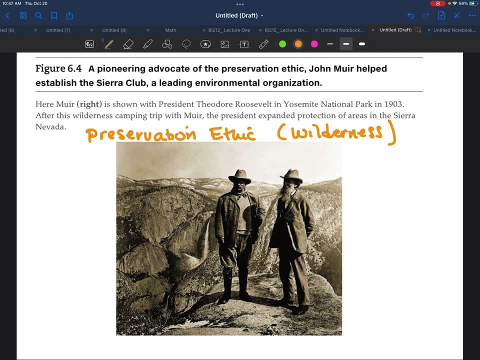 We can go into wilderness, but one of the things that we generally can't do is to drive our motorized vehicles into them, And so this would be that we need to protect the natural environment in a more pristine state, that we need to be able to drive our motorized vehicles into.